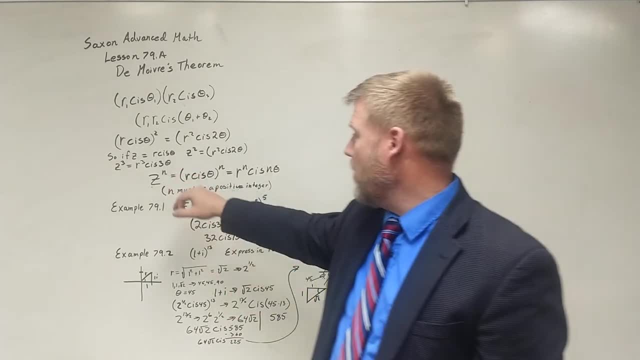 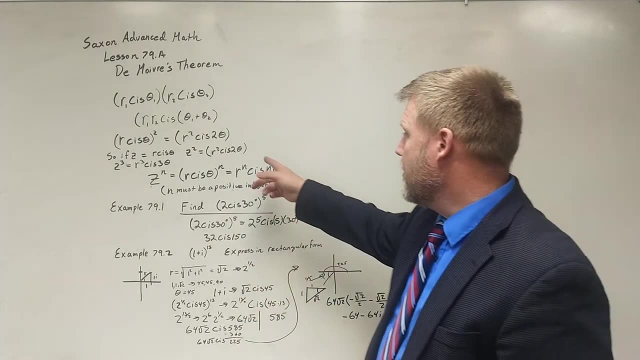 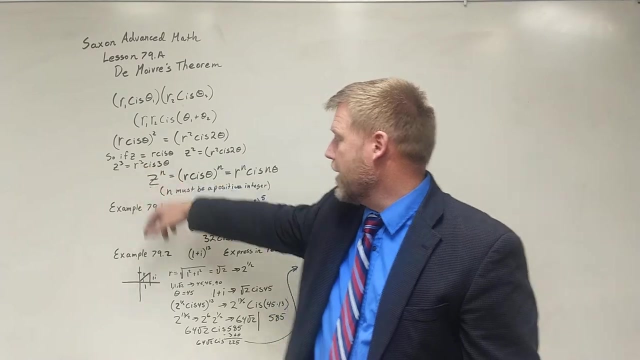 If I let Z equal R CIS theta, Z squared would be R squared CIS. 2 theta: right, Because remember, I'm multiplying the radiuses but I'm adding the angles. Well, with that theory, then Z cubed would be R cubed CIS 3 theta. 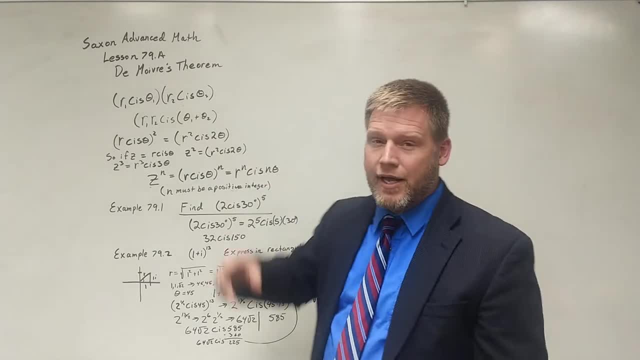 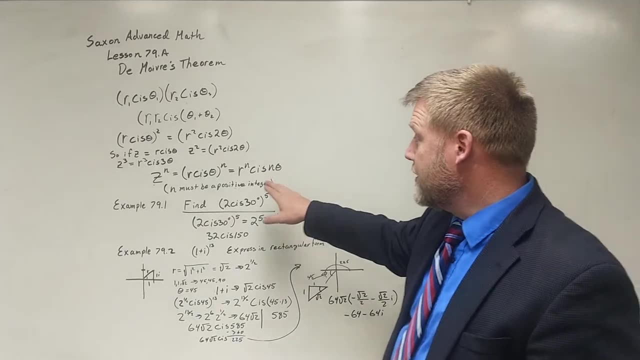 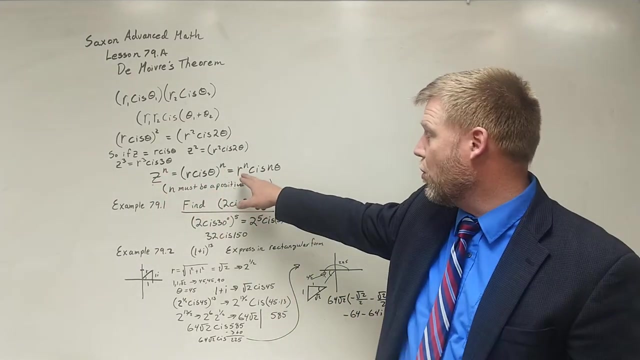 And this allows us to look at a very large set of these numbers being multiplied by each other, or squaring, cubing and so on, and realize that this works for every value, as long as n, So Z to the n equals R CIS theta to the n, which is R n CIS n theta. 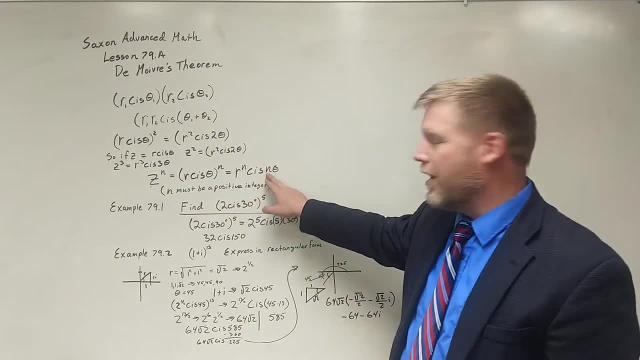 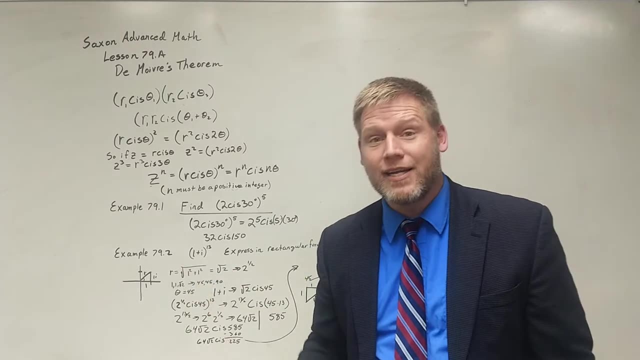 Notice that that n right there ended up as an exponent on this one and a coefficient on this one. This works only if n is a non-zero or a positive integer. Okay, It can't be a negative number. it can't be a non-integer. 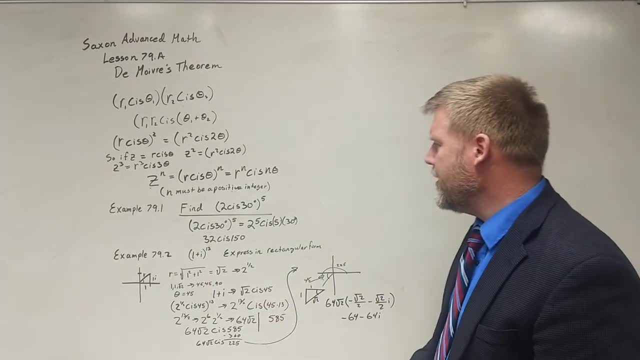 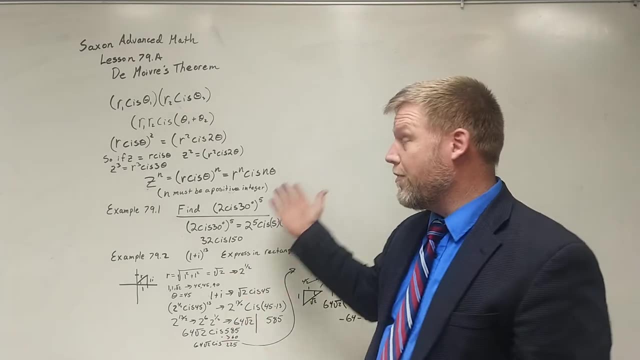 Let's look at example 79.1, and they asked us to find the 2 CIS 30 to the 5th power. Now I could write this all the way out, not using the theorem, and just say 2 CIS 30,, 2 CIS 30,, 2 CIS 30,, 5 times. 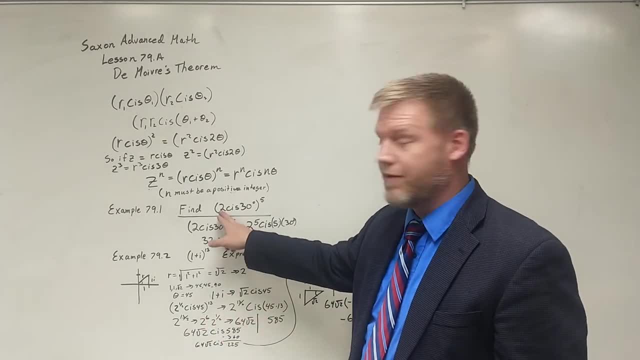 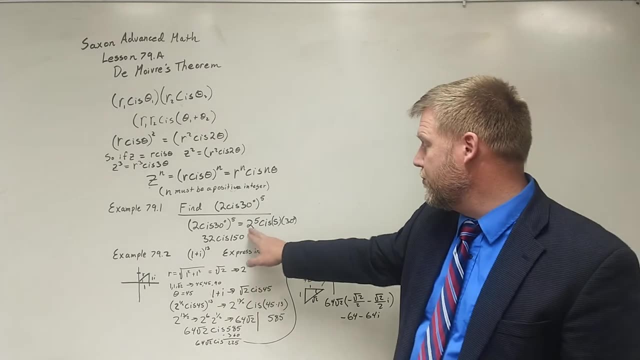 And if I did so, I would multiply every one of the 2s together 5 times, and I would add 30 to itself 5 times. Well, that sounds a lot like using this theorem, which is just 2 to the 5th CIS, 5 times 30.. 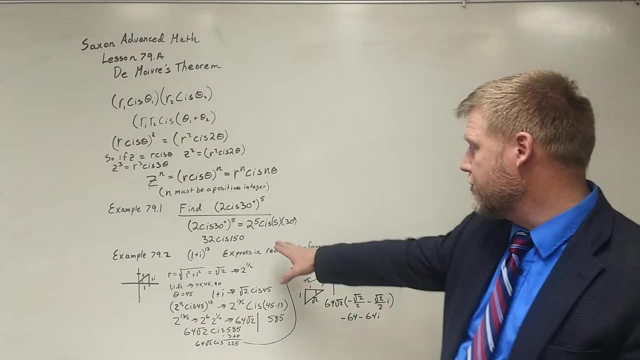 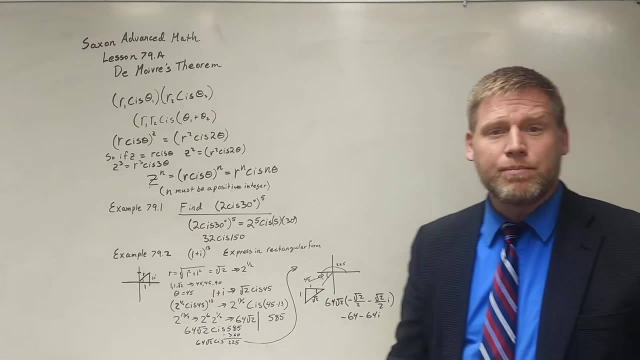 And that's exactly what I'm going to do. So 2 to the 5th, 2 times itself, 5 times is 32.. 5 times 30 is 150, and I get 32 CIS 150.. Now let's add a little more complexity to it. 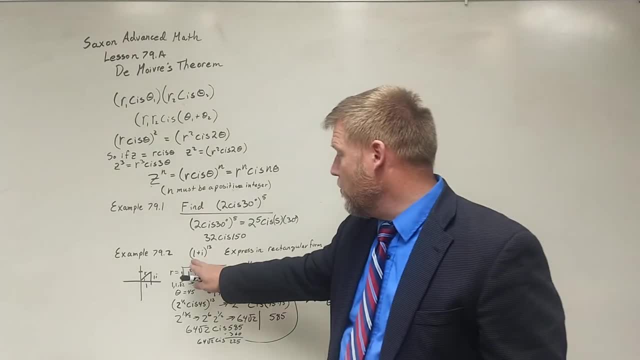 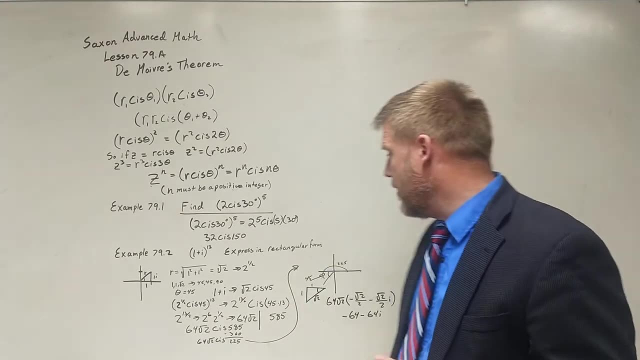 Let's say that we want to use this theorem to find out what 1 plus i to the 13th is, but we're going to express the answer in rectangular form. So what we're going to be doing is we need to convert that into polar form. 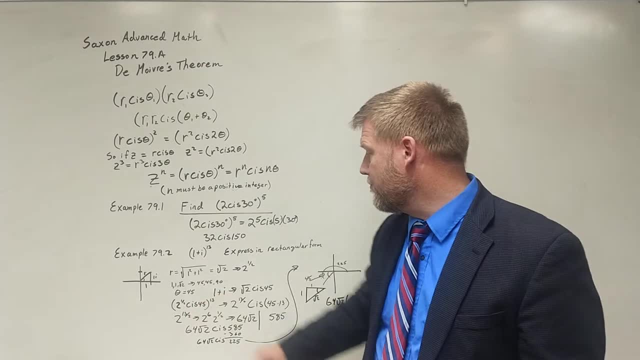 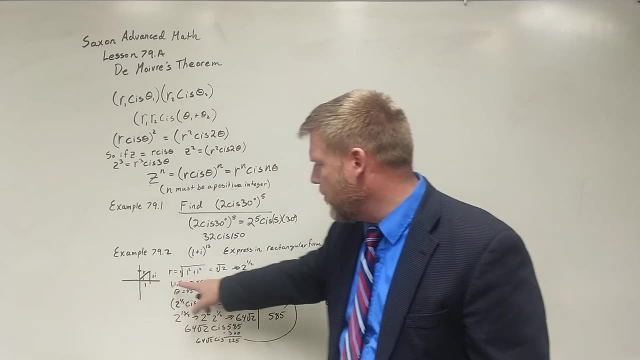 because that's in rectangular right now. Convert it into polar form first, And the way that we're going to do that is we're going to say: well, this is 1 plus 1i. So I have it on the real number line: it's over 1.. 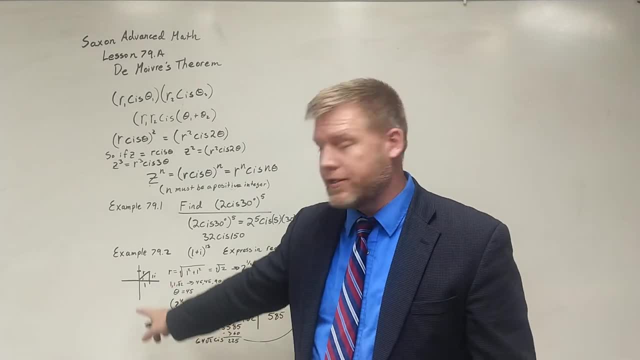 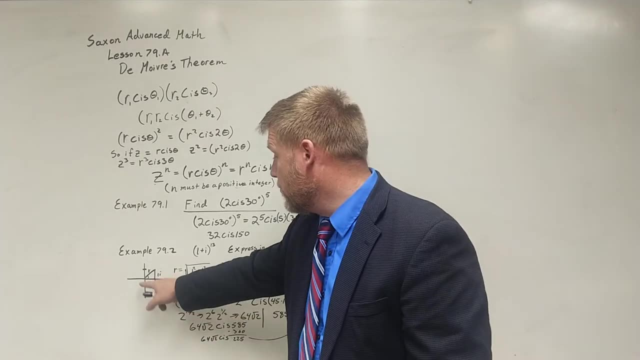 On the imaginary axis, it's up 1.. And so I say 1, 1.. Well, this is going to be a 45,, 45,, 90 triangle, right? So it's 1, 1, root 2 is that other one. 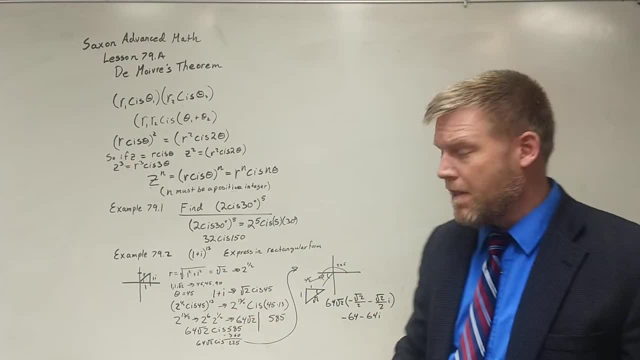 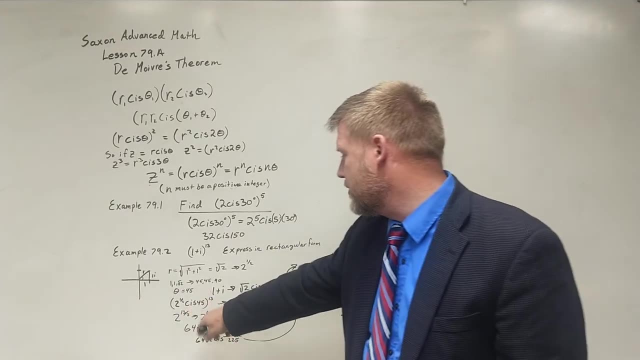 And that root 2 is our hypotenuse. When we do that we realize it's a 45,, 45,, 90. So I have it written: in the correct form would be root 2, cis 45. However, I'm going to slip in this little bit of an extra here for you. 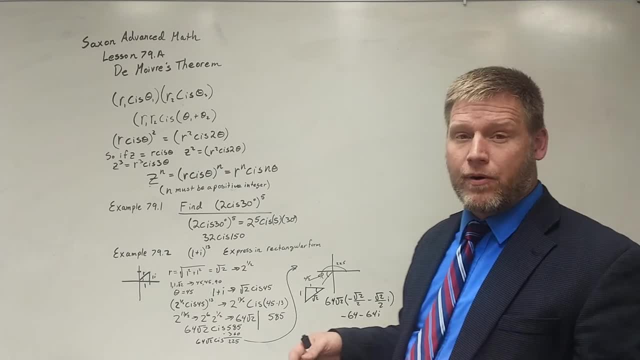 I'm going to look at it and say, instead of root 2, I'm going to write it as 2 to the 1 half power. It means exactly the same thing, but we'll see why that makes sense here in a minute. 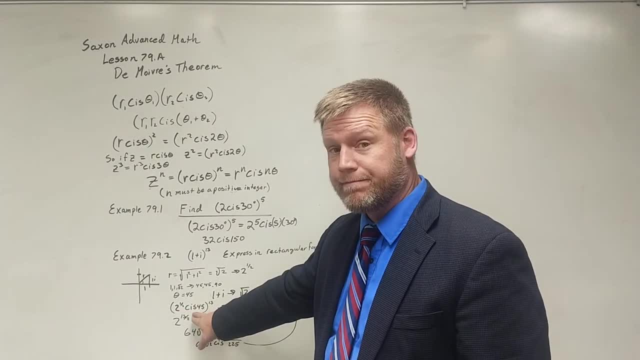 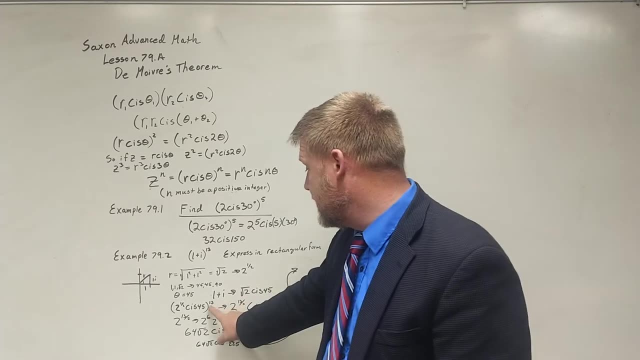 So I'm going to write this as 2 to the 1 half power, cis 45. Now I'm going to bring that to the 13th power. I can use my newfound theorem here and realize that this 13 becomes an exponent on this, so 13,. I'm multiplying this 13 over 2.. 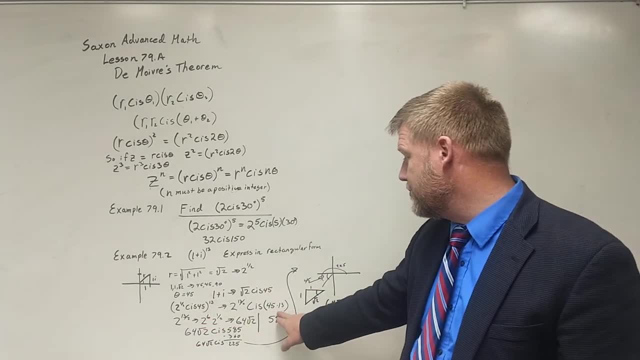 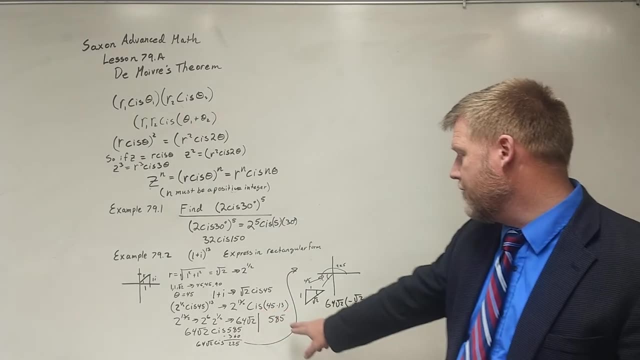 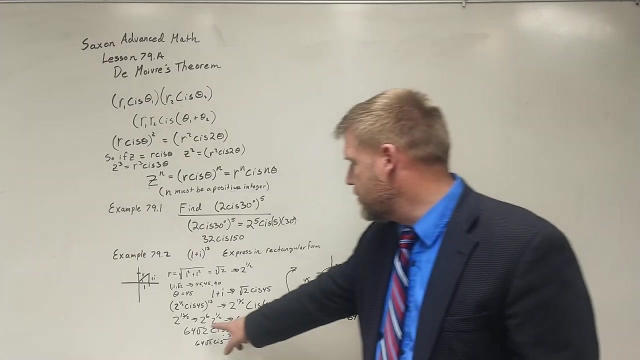 And I'm going to go ahead and say that's the same as 45 times 13.. So now I end up with 2 to the 13 over 2 cis of 585.. Well, 13 over 2 is, if I reduce that into a normal, would be 2 to the 6th and 2 to the 1 half. 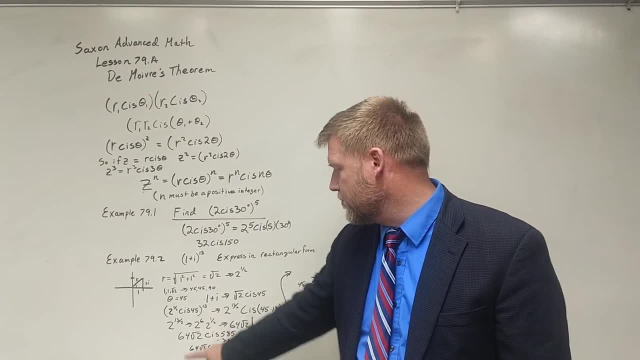 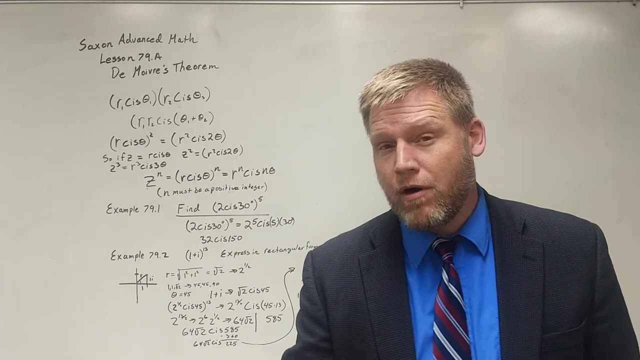 Well, 2 to the 6th power is 64, and 2 to the 1 half power is root 2.. And so I could really write this as 64 root 2: cis 585.. Now, if you remember, when we're converting from rectangular to polar, 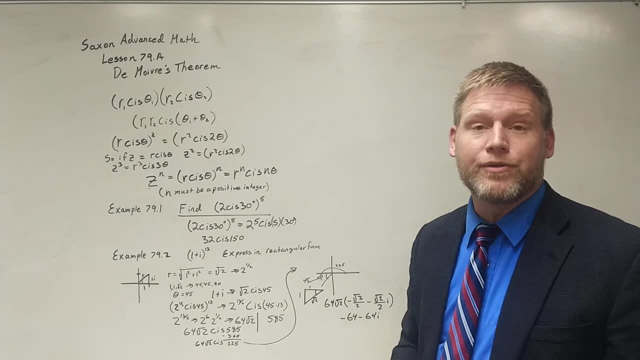 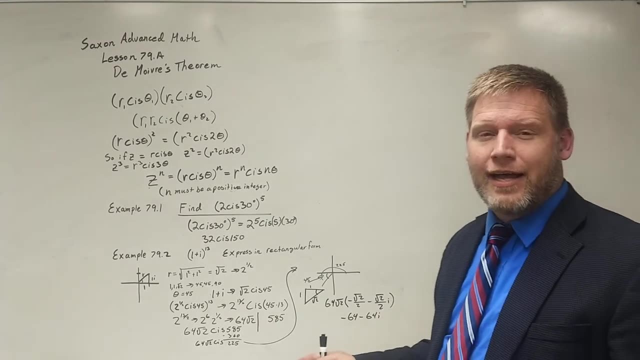 or we work with any of these. any time it ends up over 360 degrees, we can take away the 360.. If it was over 720, we would take away the 720. Because I can't tell the difference between the terminal side. 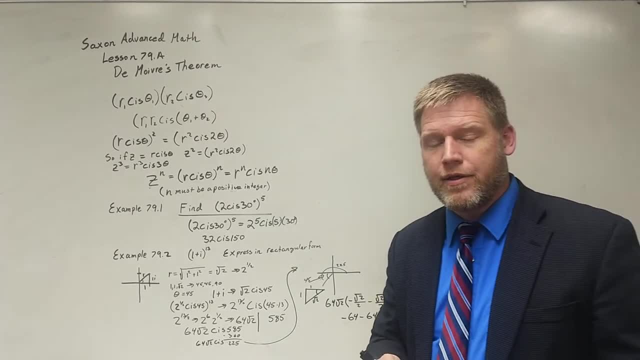 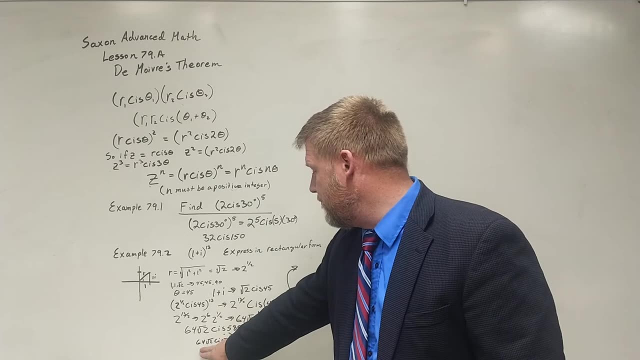 and starting initial and going around the graph there I can't tell the difference between 0 and 360.. So I can take 360 away and get 64 root 2 cis 225.. Now, normally I would be done at this point, but they asked me specifically. 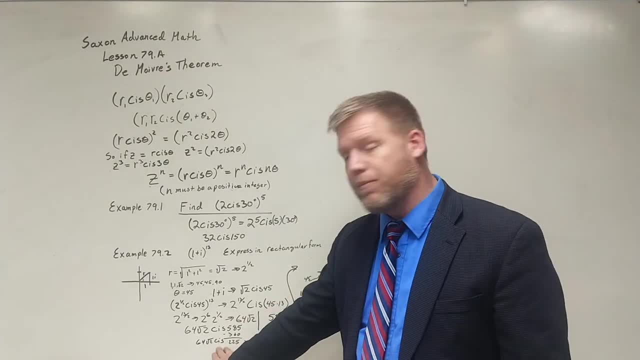 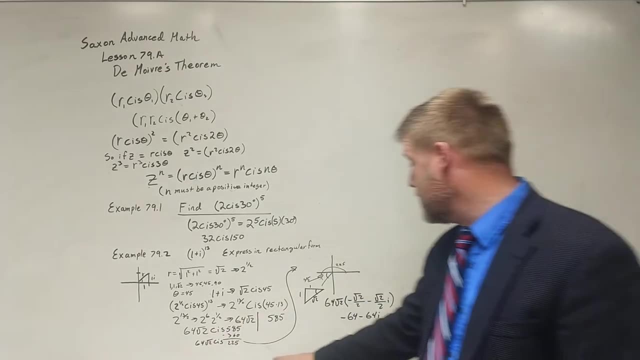 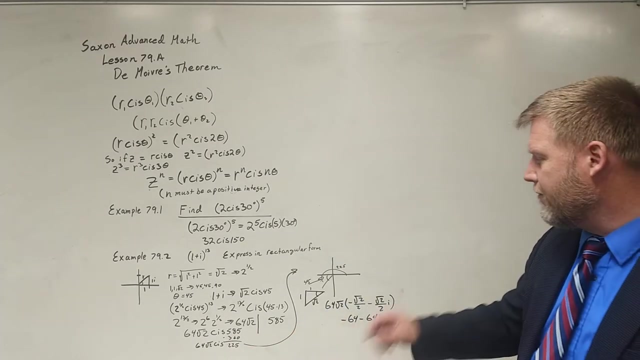 to write the answer in rectangular form. Here we are in polar format, So we're going to convert this into our rectangular format. So I put my parentheses on there and I realize that this is going to be 64 parentheses. cosine i sine of 225. 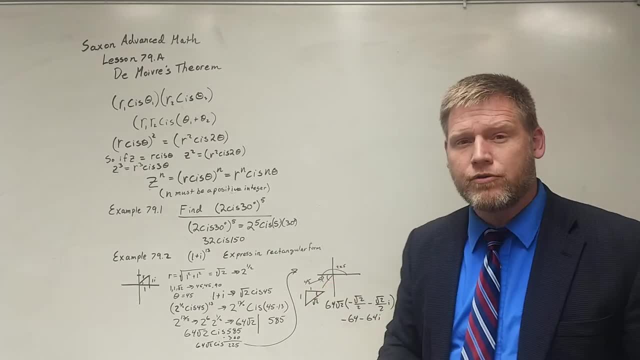 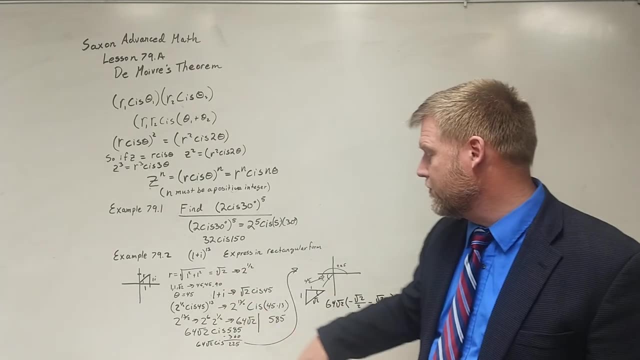 Well, 225 is going to put me into the third quadrant. A third quadrant. 225 is a 45 degree angle, which makes sense because we're finding multiples of a 45 in the first place, And that's going to be a 1: 1 root 2.. 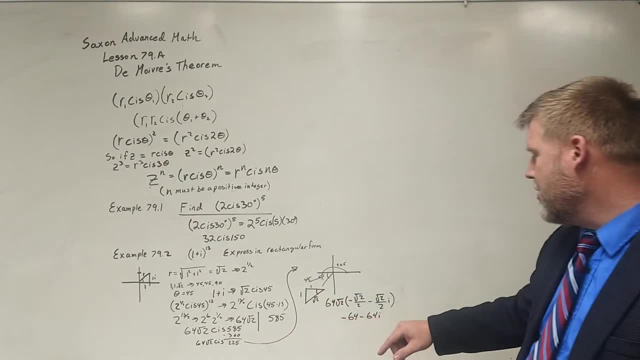 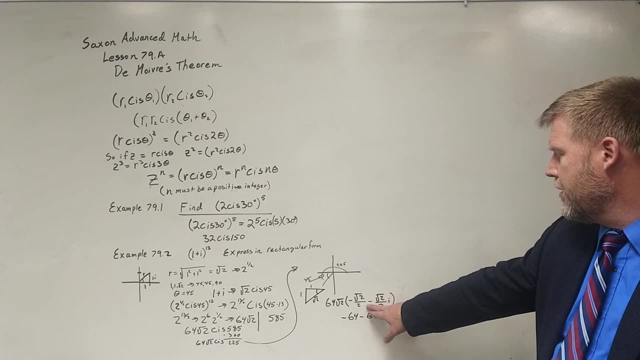 Well, so the cosine i sine right Cosine is going to be adjacent right over hypotenuse, And when I simplify that, that makes it root 2 over 2. And it is negative. Remember all students take calculus. 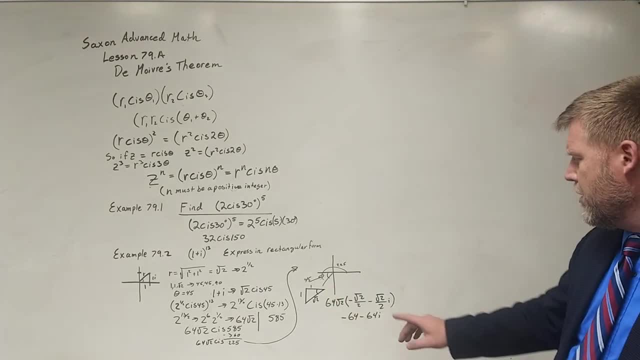 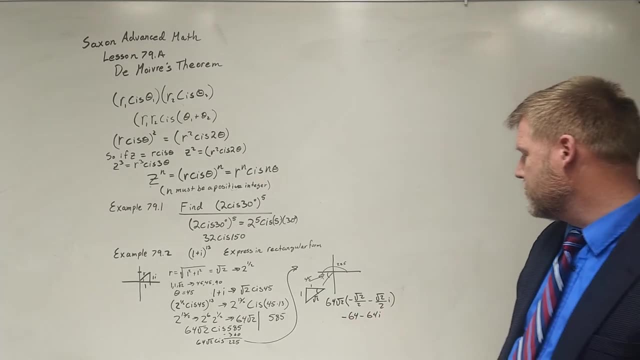 So the only thing positive in the third quadrant is the tangent. So there's my conversion for the cosine plus the i sine, the sine root, 2 over 2.. And that's going to give me that same, because it is a 45-45-90 triangle. 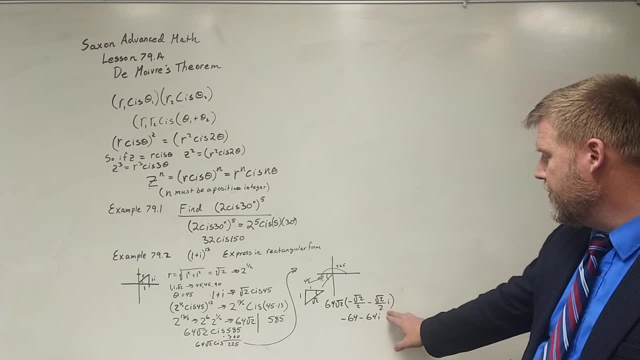 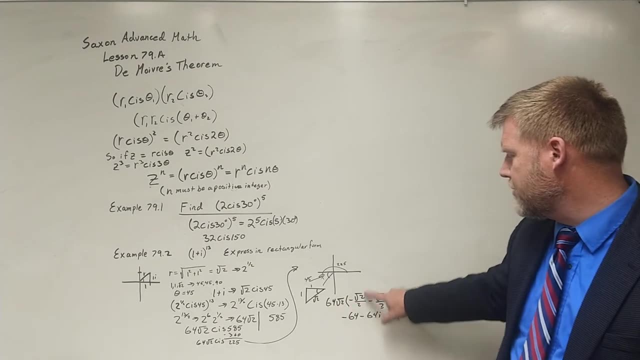 it's going to give me. the sine and the cosine have to be the same. It's also negative in the third quadrant. Then I go ahead and separate this and put 64 over 2 times a negative root. 2 over 2 reduces to 64.. 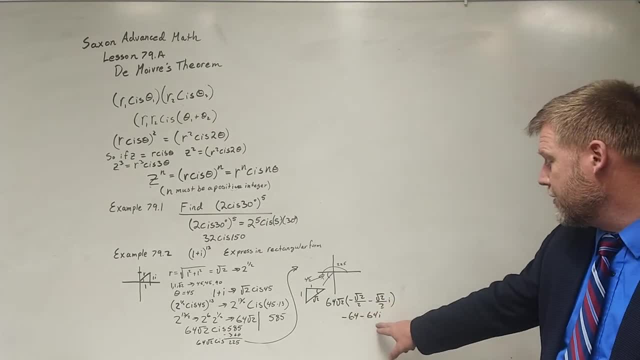 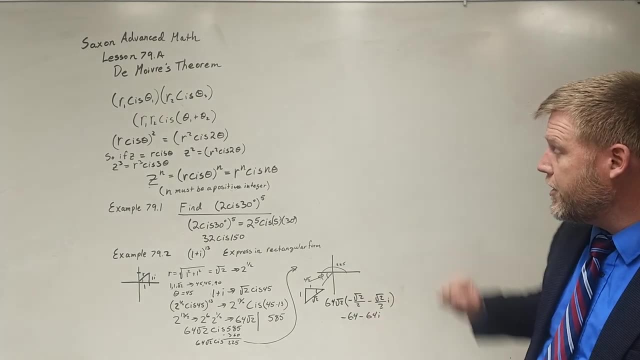 64 root, 2 times a negative root, 2 over 2, and that's going to give me a negative 64i. And that's my answer. And that's how I use this format, this theorem, to convert it from rectangular to polar. 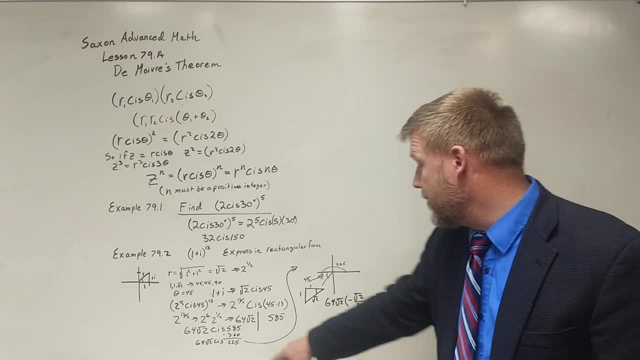 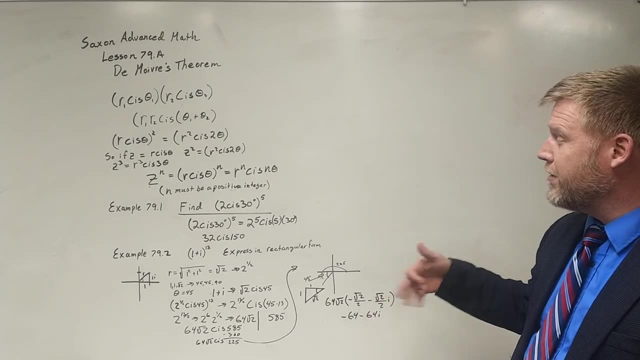 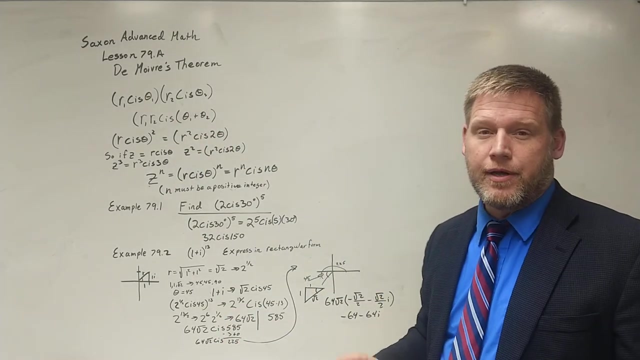 use the theorem de Morville's theorem, end up with it in polar format and then convert it back to rectilinear format for my answer. So this is a theorem that can be used any time I have multiples of the same cosine i sine polar format being used.